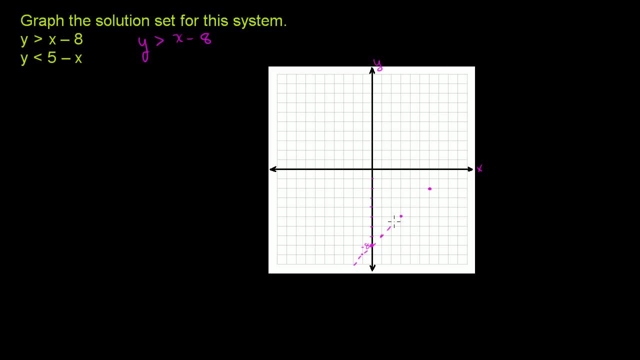 dotted line. I'll do my best to draw a dotted line, which is surprisingly easier to draw than a non-dotted line. So that is essentially a dotted line. version of y is equal to x minus 8, but we're going to be greater than that. 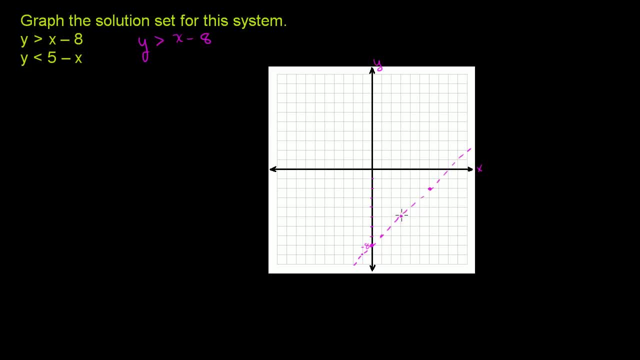 So for any x, x minus 8 is going to be on that line, but the y is going to be all the values greater than that. So you pick any x, this is x minus 8, the y value is going to be all the y's greater than that for that x. 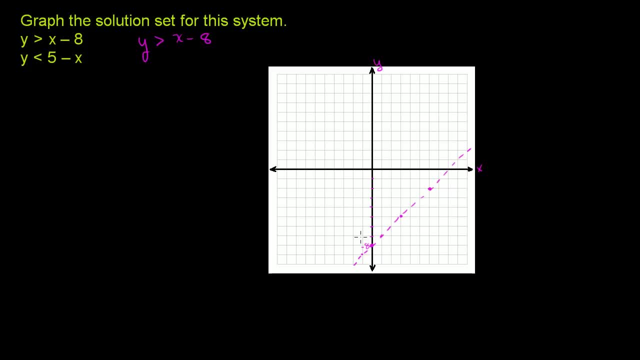 So the solution set for y is greater than x minus 8 is all of the area above this line and it doesn't include it and that's why I put a dotted line there. So let me do that in a lighter color. So it's literally all of this area up. here is the solution. 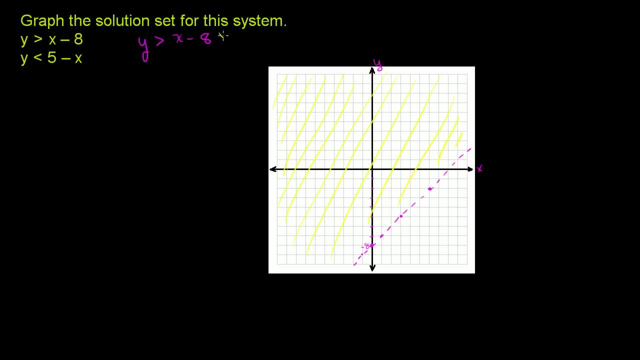 set for this first inequality. Now let's do the second inequality. I'll do it in another dark color We have: y is less than 5 minus x, or we could write that as negative x plus 5, so it looks a little bit more like our. 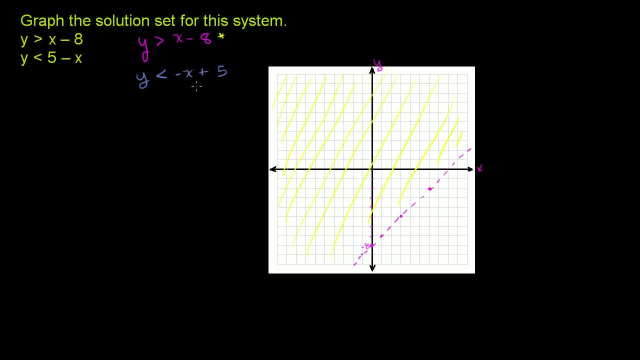 slope-intercept form Now. Now, If we were to just graph: y is equal to negative x plus 5, it would look like this: We'd go in the positive y direction: 1,, 2,, 3,, 4,, 5.. 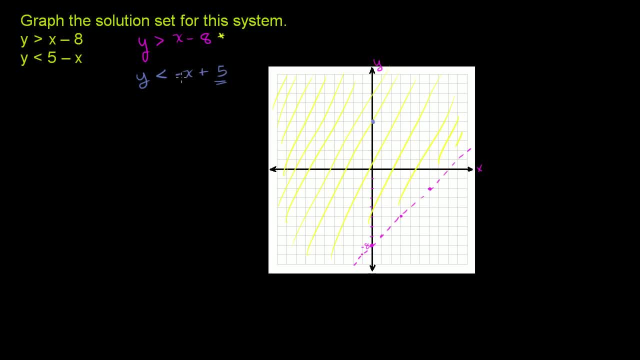 That is the y-intercept right there and it has a slope of negative 1.. So if we move 1 in the x-direction, we move down 1.. If we move 3 in the x-direction, we're going to move down 3.. 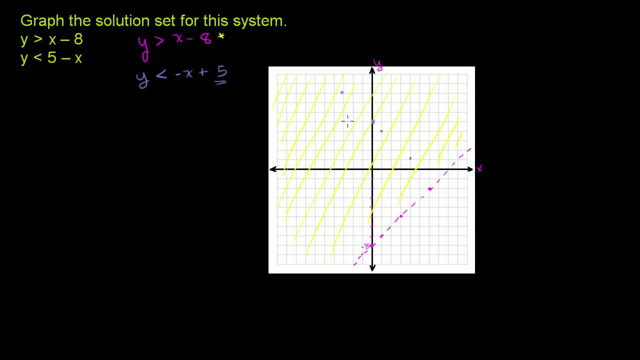 If we move back 3 in the x-direction, we're going to move up 3.. So this line is going to look like this, And I'm going to do it a dotted line, because we're not including it. It's not less than or equal, it's just strictly less than. 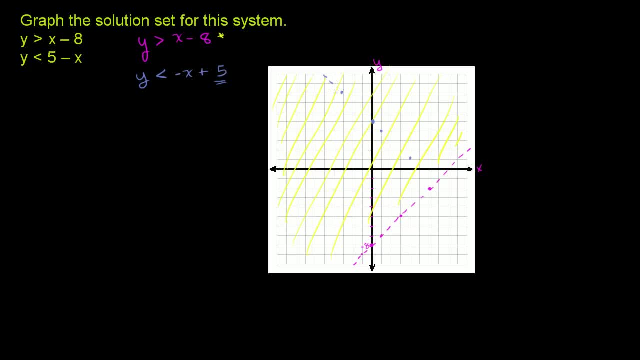 So it won't include the line. So it's going to look something like this: Try my best to draw it as neatly as possible. I think that is a respectable job. This is the dotted line version of y. is equal to negative x plus 5.. 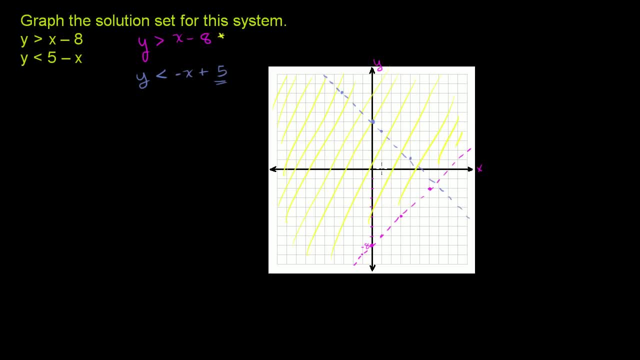 It's dotted because we're not including it Now for any x you pick an x. let's say x is equal to 1, negative x plus 5 is going to get onto that line. But for that x we only care about the y's that are less.